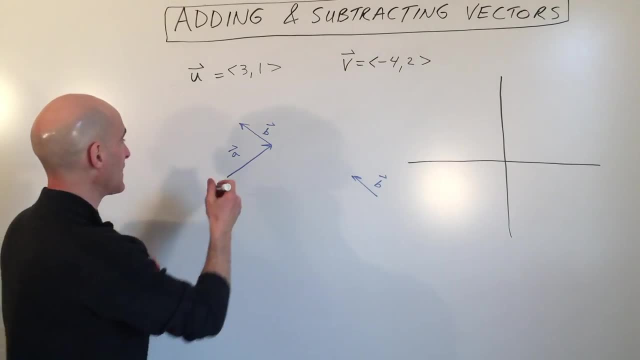 resolved of those two vectors being added together, is this vector right here: a plus B, that's the resultant vector of adding together. so it's kind of like if you were to walk this direction and then walk this direction, the end result is you could have cut through the backyards of your friends and gotten. 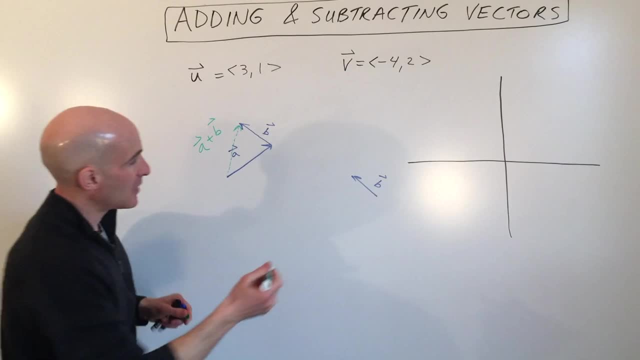 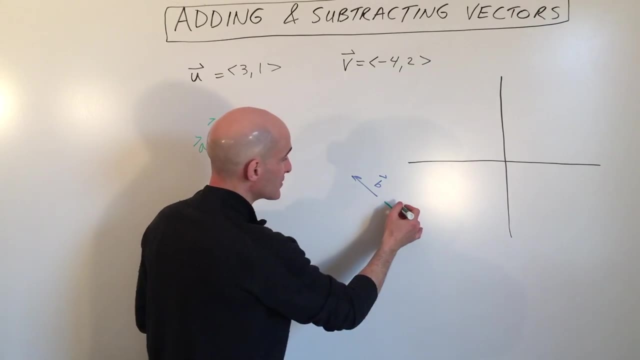 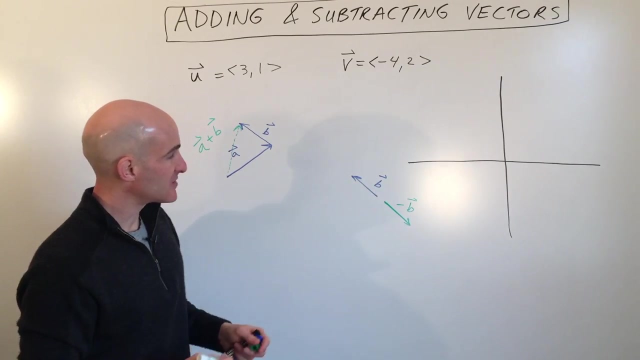 there a little bit quicker. okay, now if you subtract vectors. okay, when you subtract a vector, what it means is that the vector is going about 180 degrees the opposite direction. so this vector here would be negative B. same length, 180 degrees opposites, point in the opposite direction, that's a negative B. and so now if we 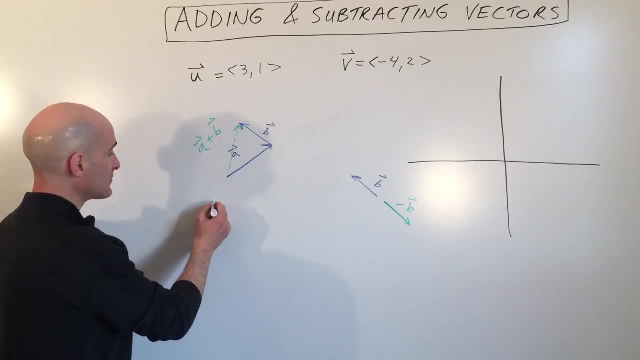 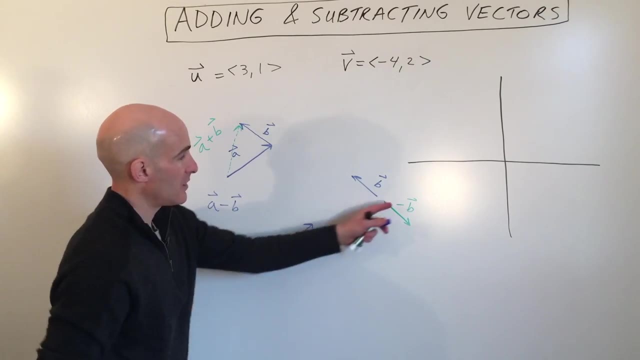 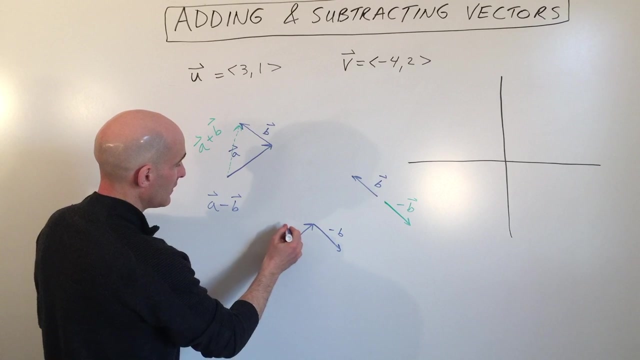 wanted to do this again. let's do a minus B this time. okay, a minus B. so vector a is here, negative B is going this direction now, okay. negative B is going in a greater pattern. okay, and another 50 degrees. where one ends, the other one begins, and so our end result is that vector right. 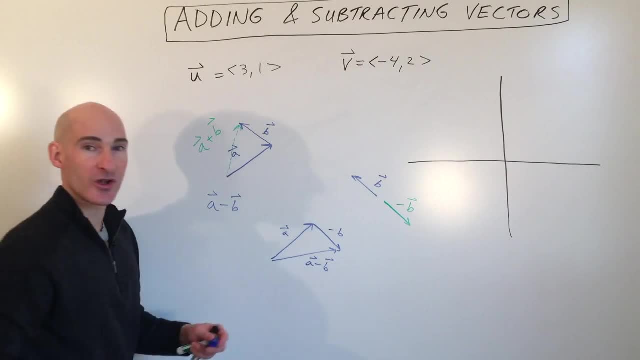 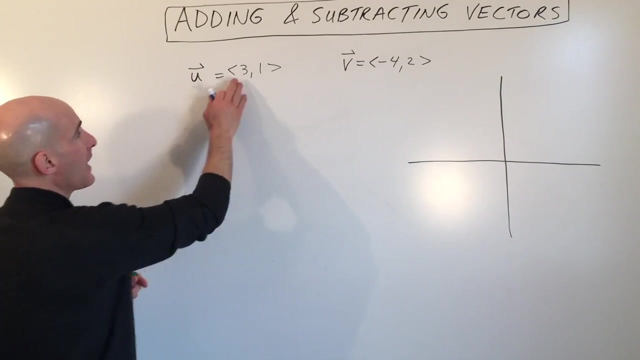 there a minus B. that's what they call the resultant vector. so this has been a little bit about how to work with the vectors, just just with the drawings we can. now let's look at that, the algebra part of it. how do you add, subtract and multiply vectors? well, all you have to do is add the X components and add the Y. 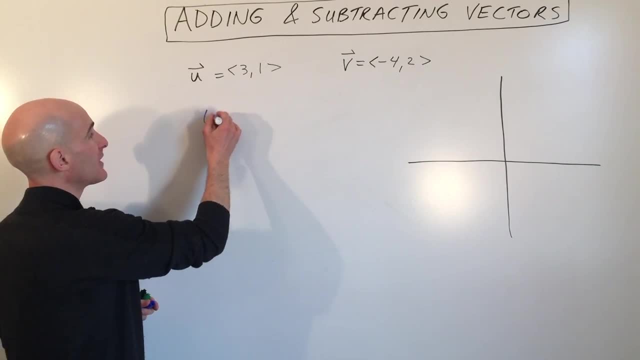 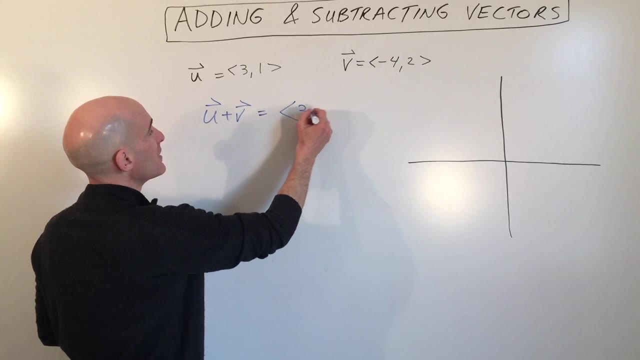 components or subtract X components, subtract the Y components. so if we want to find out what u plus V okay is, in this example, we just take 3 plus negative 4 and 1 plus 2. so I'm just adding the X's and I'm just adding the Y's and 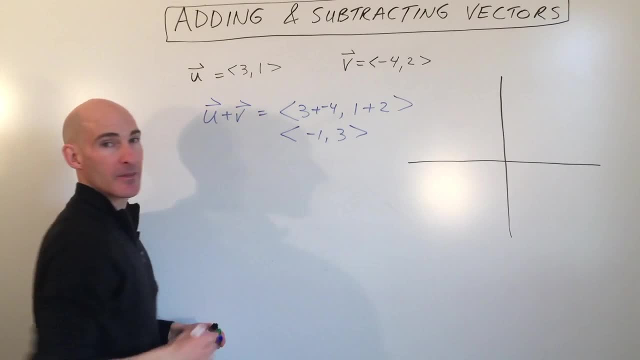 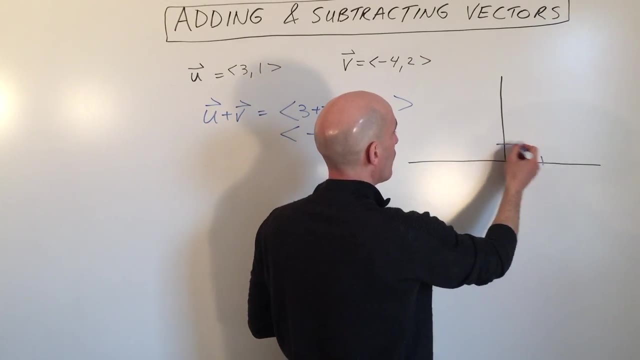 that's going to give us negative 1- 3. so that's the end result. and if you want to see what it looks like over here in the plane, we've got three: one okay, so that's vector U okay, and vector v is negative 4- 2 okay, so we're going left 4. 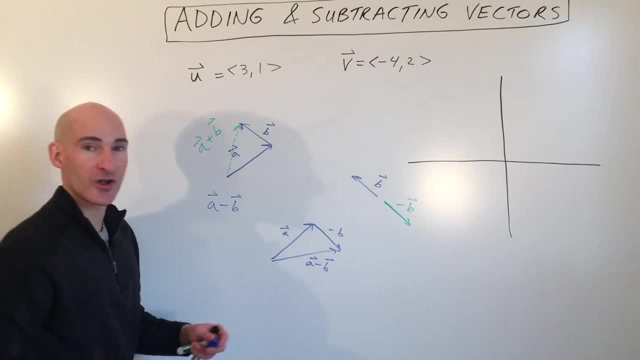 there a minus B. that's what they call the resultant vector. so this has been a little bit about how to work with the vectors, just just with the drawings. okay, now let's look at that, the algebra part of it. how do you add, subtract and multiply vectors? well, all you have to do is 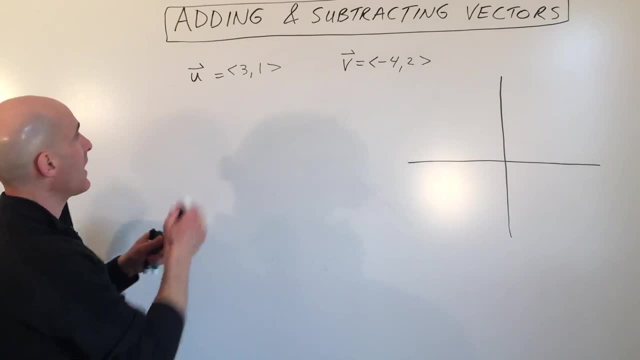 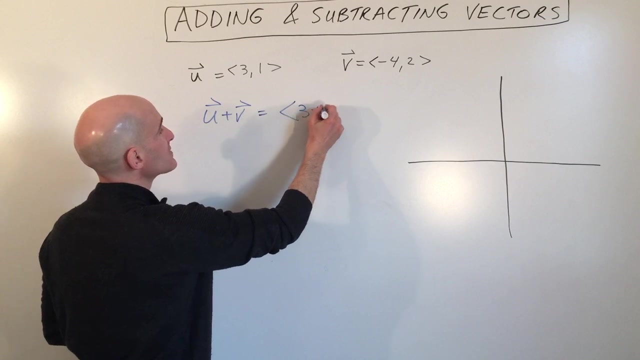 add the X components and add the Y components, or subtract X components. subtract the Y components. so if we want to find out what U plus V okay is, in this example, we just take 3 plus negative 4 and 1 plus 2. so I'm just adding the X's and I'm just adding the Y's and that's going to give us negative. 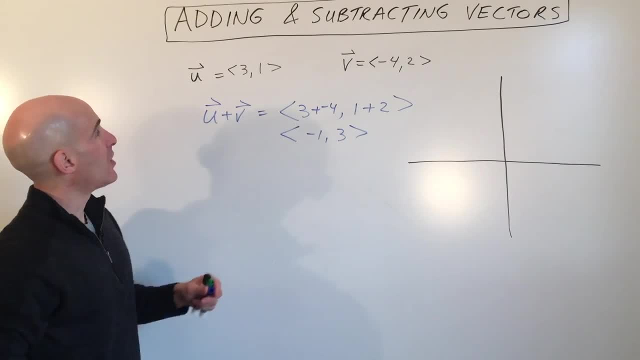 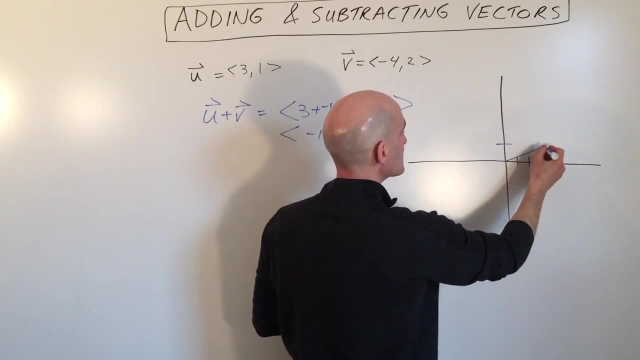 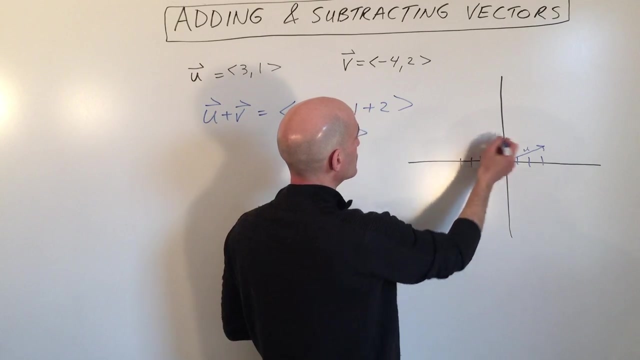 1- 3. so that's the end result, and if you want to see what it looks like over here, you can see that the we're here in the plane. we've got 3- 1- okay. so that's vector U okay and vector V is negative. 4- 2. 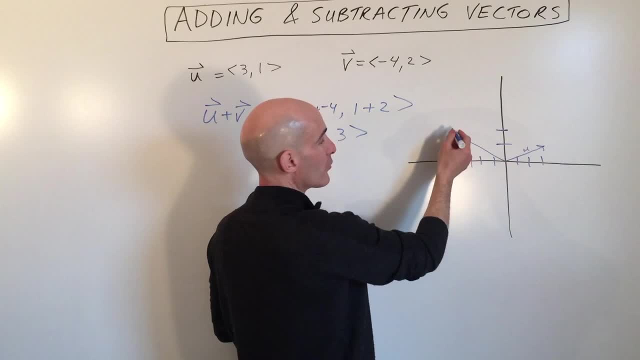 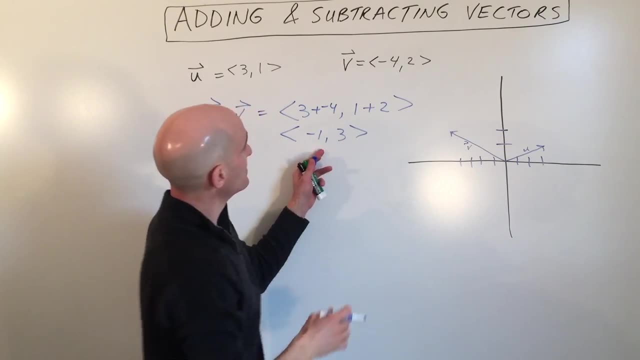 okay, so we're going to left 4, up 2, and that's vector V, and so now what we're going to do is we're going to. the end result is negative 1- 3. so it's negative 1- 3. okay, right there. 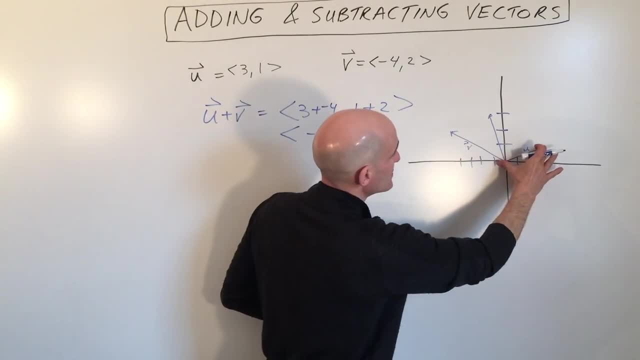 that's the end result. now, remember, you can take these vectors, you can slide them left and right, up and down, you just don't want to rotate them or make them longer. so if I shift this over and shift it up, see, there's vector U. okay, where one terminates, the other one begins, and you can see. 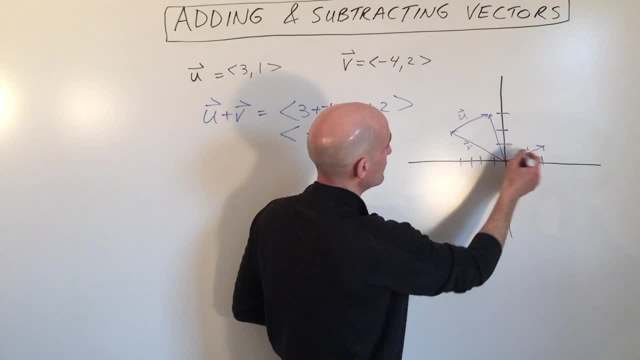 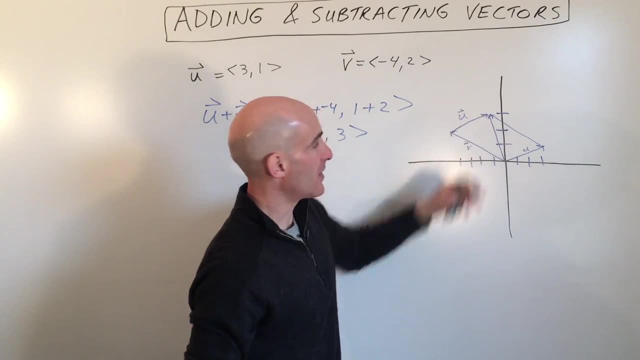 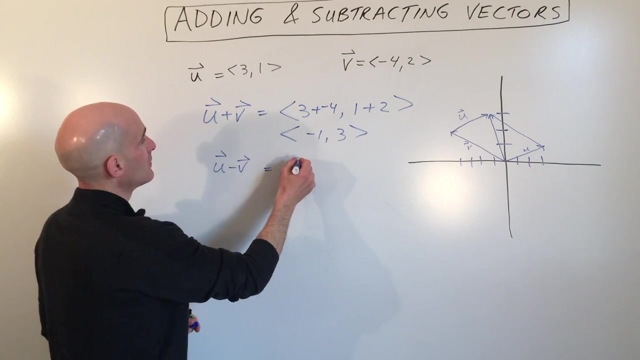 the end result is this diagonal here: same thing with vector V. you could shift vector V over here, okay, and the diagonal is the end result of adding those two vectors together. okay. now, if you do the same thing, U minus V, that's going to be 3 minus negative 4, and 1 minus 2, which is 7 and negative. 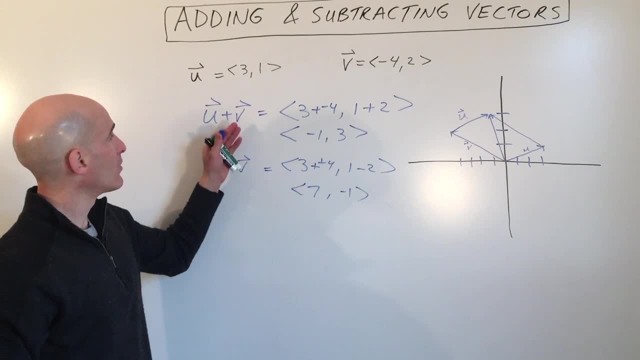 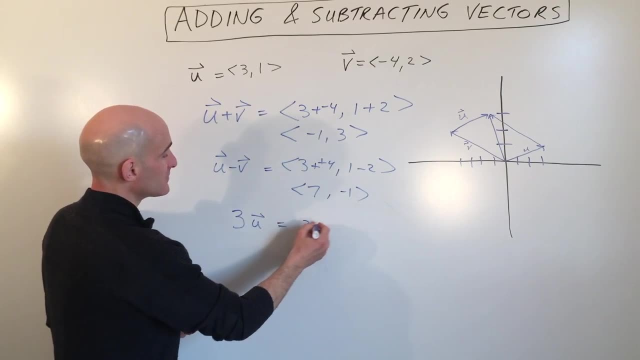 1, and then the last thing I'll show you is that let's say you want to multiply by a scalar, like they call the scalar multiplication 3 times U. all you have to do is multiply the x and the y components by 3, so it's just like doing the distributive process.